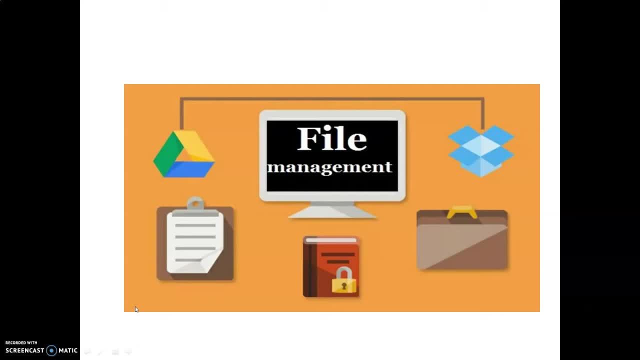 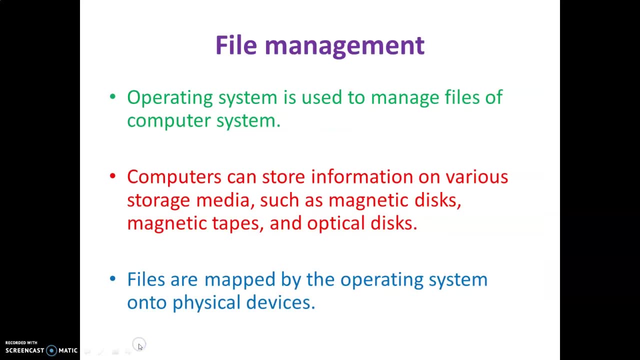 read the content of the file. So this is basic information regarding the file management. So let us start File management. The operating system is used to manage files on the computer system. Basically, computers can store information on various storage media. I told you like we are having the magnetic. 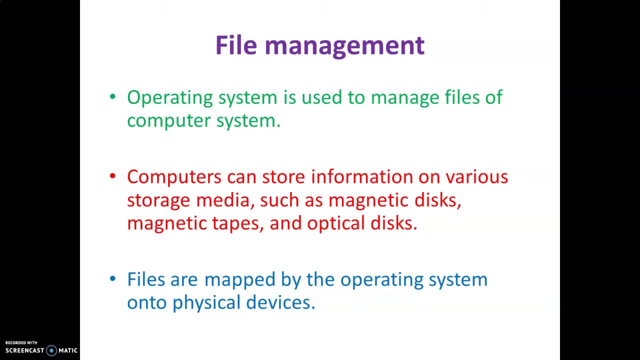 disk, magnetic tapes We are having, optical disk We are having. So why we are storing all these files on these particular different devices, so that these files can be mapped by the operating system on physical devices. So what are the Files Goals of the file management? So the goals of file management are to keep the track of 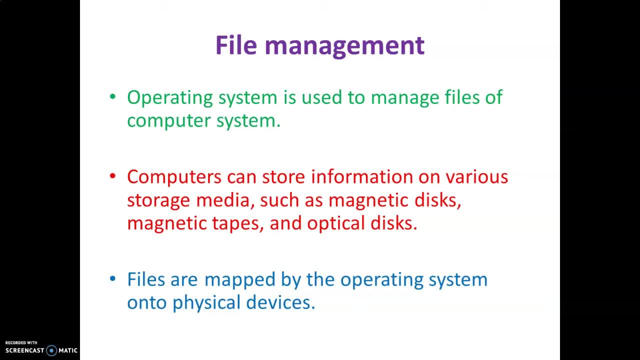 all the files and the folders, like so many files and folders, are available in the system. So our operating system is going to keep track of whatever the newly created file exists or if the already file, any type of operation has been done on the file, like creation, deletion. 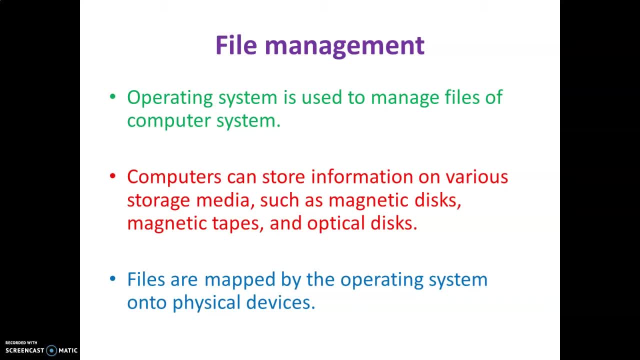 modification. So it is going to keep track of each and every operation which is done on the file file or the folder. Next is it is going to allocate the space to your running program, That is, it is going to allocate the space to the process on the hard disk. So if you are writing any program, 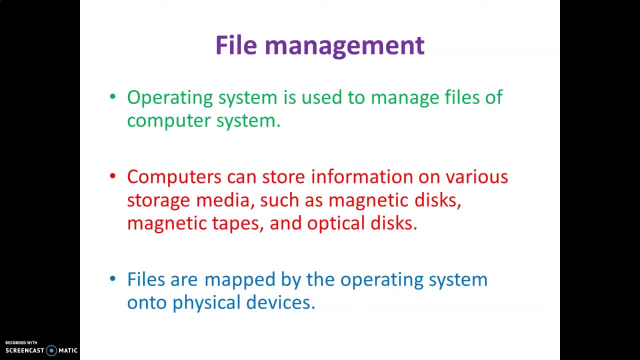 any C program or any C++ program. it is also going to allocate the space to your running program, And that running program is Known as your process. Third kind of aim of the file management we are having is it is going to allocate as well. 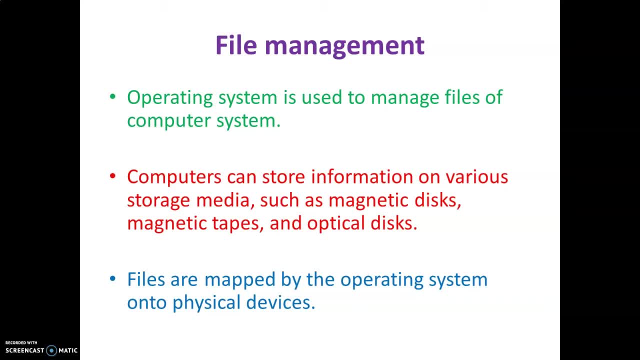 as de-allocate the space to and from the file as well as the folders. So whenever you are creating some new files and folders or if you are deleting any already existing file and folder, so whatever the space has been allocated during the creation, So after the deletion, 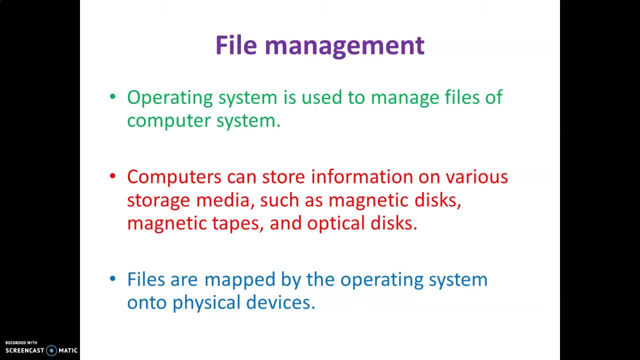 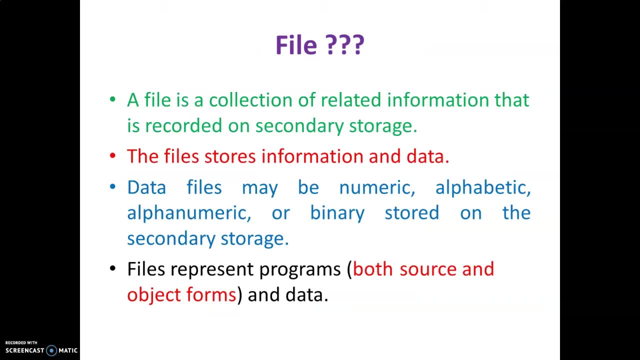 That space is going to get free. So these all are the different reasons why we are managing the files in the system. So so many discussion has been done on the files. So let us see the formal definition of the file. So what is file now? 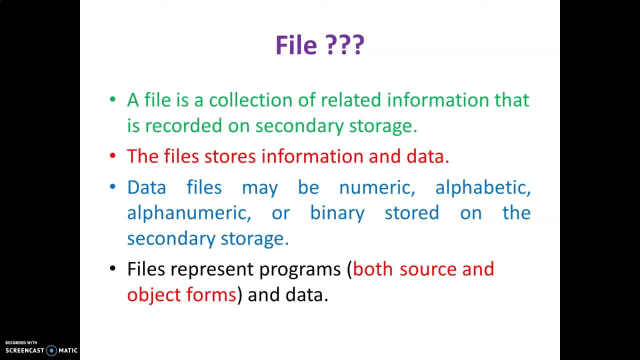 So file is a type of a collection of related information that is recorded on the secondary storage. So there are so many in today's market. There are So many different files are existing, Like if I talk about there are document files, are there video files, are there audio files. 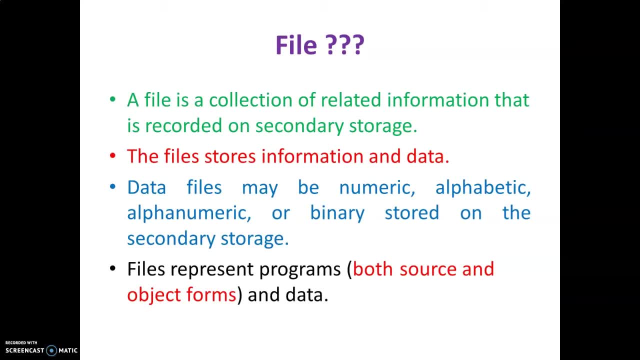 are there images, files, are there? So so many files we are storing on our secondary storage devices. So these files are going to store the information as well as the data. So data files, when we are storing it can be your numeric data, alphabetic, alphanumeric. 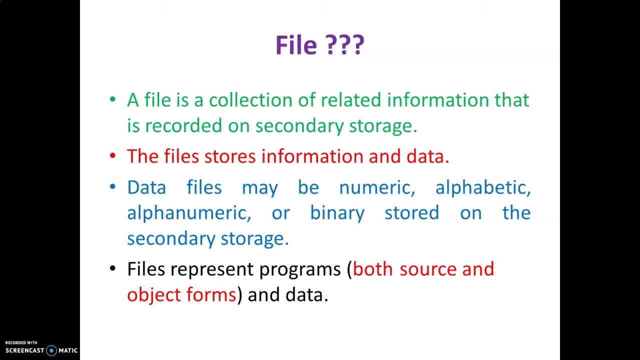 binary, So any kind of data So many people are storing in your files. So files are also represented in the form of programs like the C program, when you are writing the source code And after that you are converting that source code into the object forms. 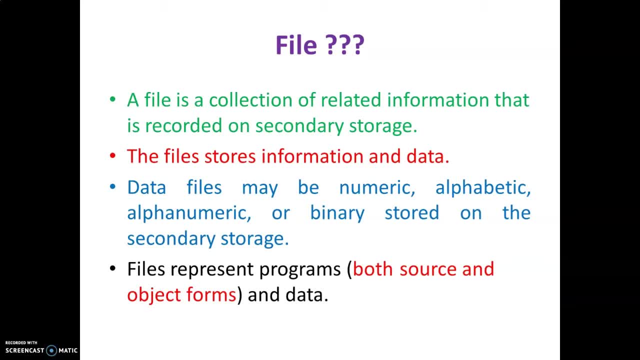 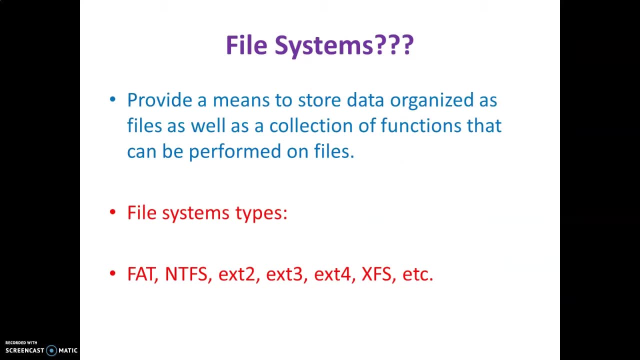 So these all are the different things which are available related to the file. Then what are the file systems? So file system provides means to store the data in an organized way. So the organization Of all these files basically is done by the file system. only means that, whatever the particular 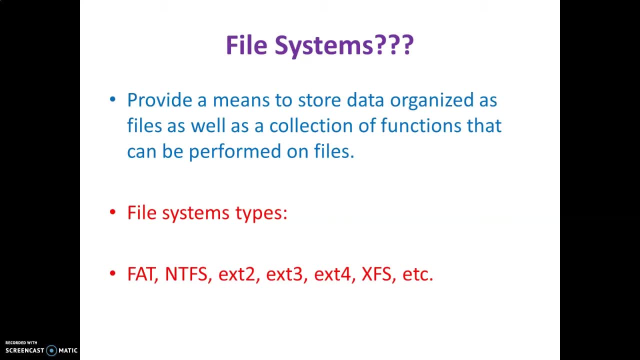 name you are giving, whatever the particular location you are giving. So each and everything you are organizing in such a way so that if operating system is going to find any of the file in future, it can be easily accessed. So this is a reason why this file system has been used. 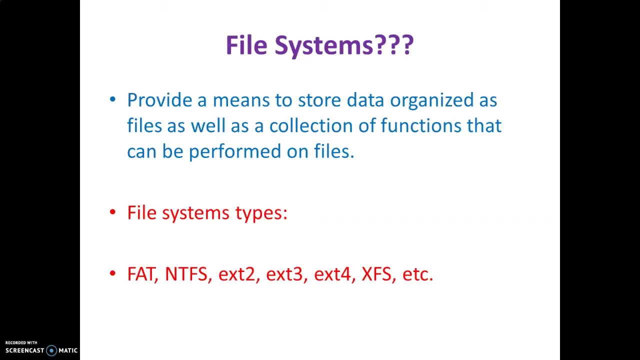 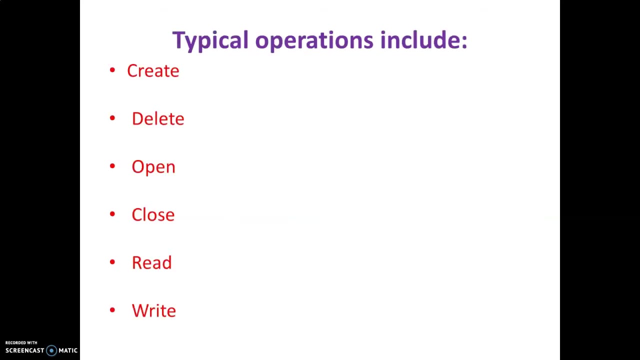 So If systems are providing different types of file system- some of the examples I have already mentioned, like FAT, we are having NTFS, we are having then EXT2, EXT3- so many different file systems are existing today- Then we are having what are the different type of operations which can be done on the 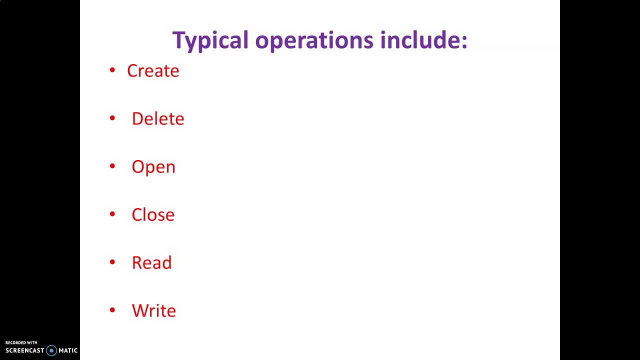 files. The very first operation is creation, or you can say creating a file. So It is very simple, if you are talking about the Linux operating system, how we create the files, like using touch command, or you can say using mkdir, we are creating the directories. 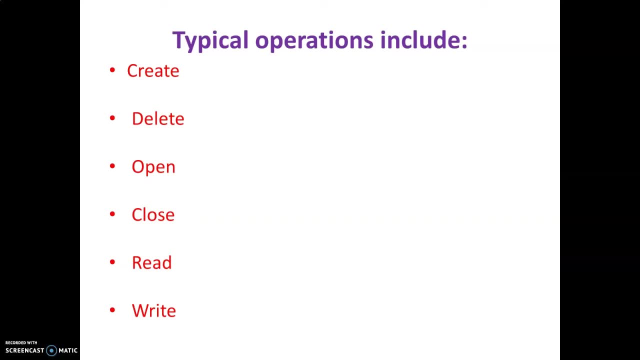 or with the help of Vim editor, we are creating again the files. If you are talking the Windows operating system, like, we know how to create the folders, like right click, right click with the mouse, you are getting the folder option. So what you are doing? all with all these things, you are actually creating the new files and 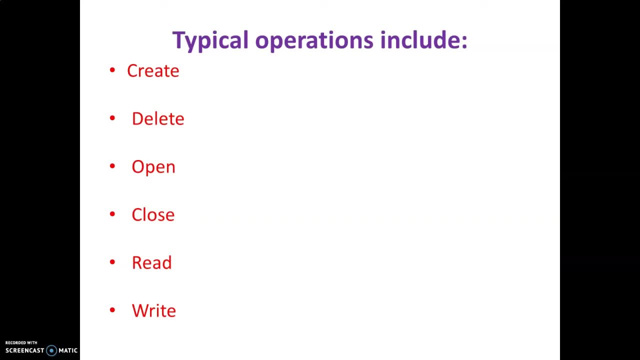 allocating the space in your system, Then we are having is the deletion. so whatever the files you have created, you can also delete them. So why you are basically deleting them? because to release the space which was occupied by those particular files. Then the next type of operation we are having is opening. 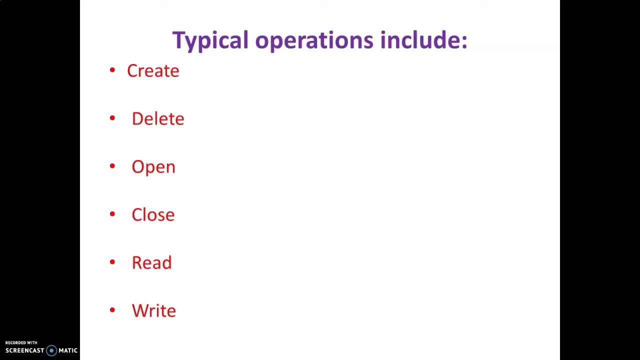 So if the folder is there or if the file is existing with the help of double click or you can say You are opening that particular file to view that or to read the content of that file or the folder, Then we are having is the close, whatever the file has been open. 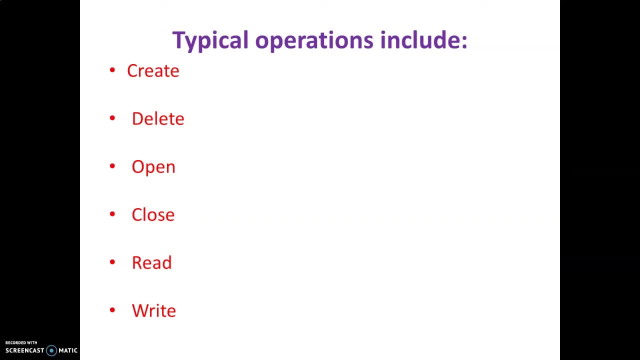 You can close very. you know how to close this, So so I think very easy operation we are having how to close this particular file or the folder Then we are having is the reading operation. So what is this reading like in the case of privileges? 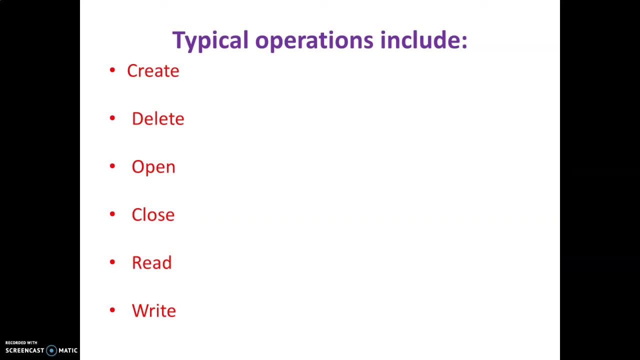 Also We have done so. not all the users are having read and write operations, like if, in the case of read, the user can only view the data means he is only able to read the content within the file, Then we are having the writing. writing means doing any modification or altering the content. 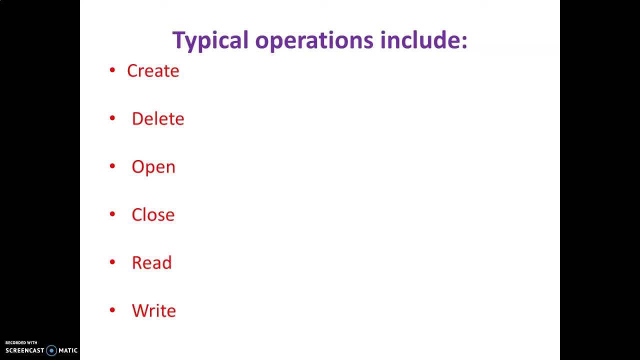 inside the file. So this is all the operation. other than that we are having like copy operation We are performing. then we are doing any renaming part we are doing. So other operations are also included in the case of fights. The next topic we are having is the file attributes. 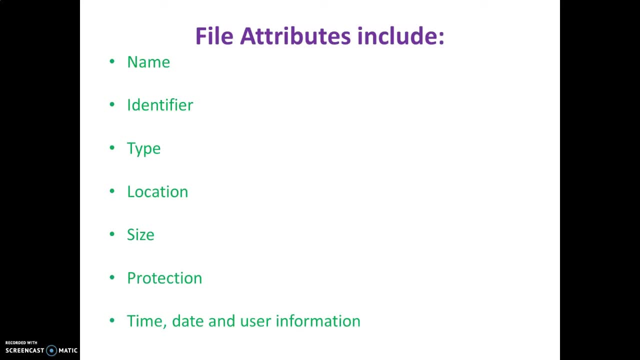 So what are the different types of attributes, attributes available related to the fights? The very first one we are having is the name, So the name, whatever the name, which which will be the human readable form, Like, whatever the name you are giving, suppose, if the file is related to the 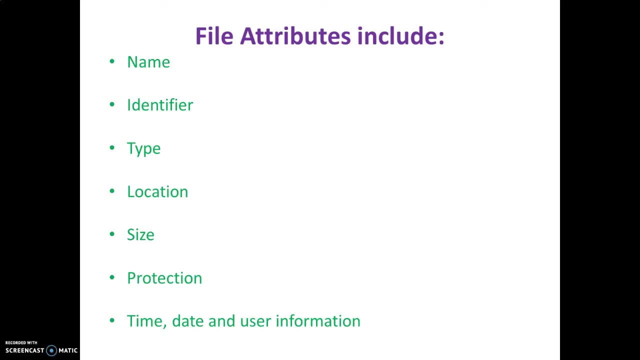 Any document, suppose ABCD, ABCD, dot, DOC, like dot, TXT, with the extension you are giving, So any human readable name you are giving to your files, So it can be the collection of any characters, Then we are having the identifier. So throughout the system there are so many files which are existing. 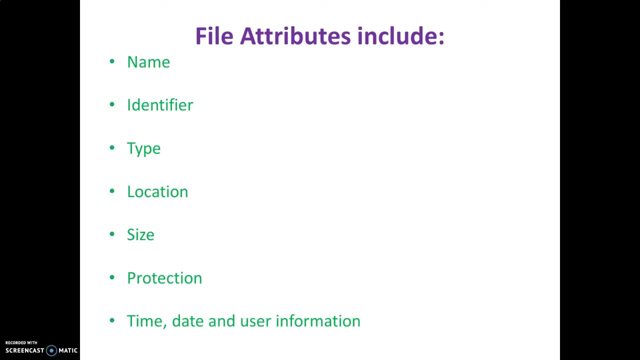 So how these all files are Differentiated with the help of those unique numbers only, like Any uniquely numbers we are giving to our fights so that they can be differentiated from the other fight. Then we are having the type. So, basically, type is needed for the system that supports different types, like so many. 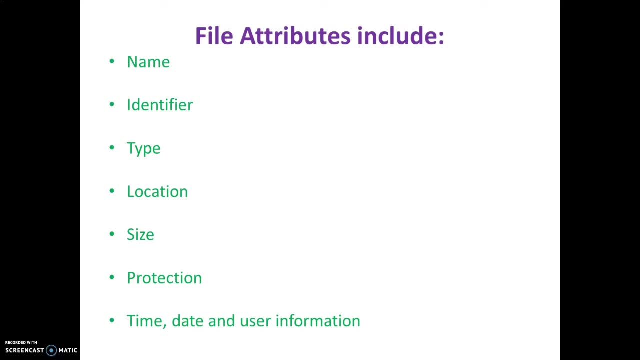 different type, I told you, for the video type is different, video file type is different, for the audio file type is different, for so many types are there. Then we are having the location, Providing the location where we are going to store that particular file. 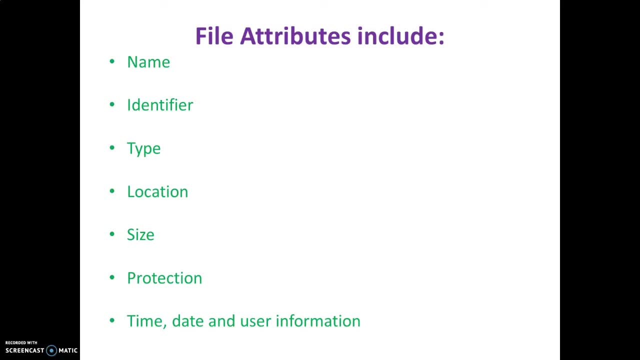 Then is the size. So size can be in the bytes, in the words or in, or in the case of blocks, for whatever the current size of the file which you are storing in your system and protection, You can also give the protection some privileges. you can provide access, control information. 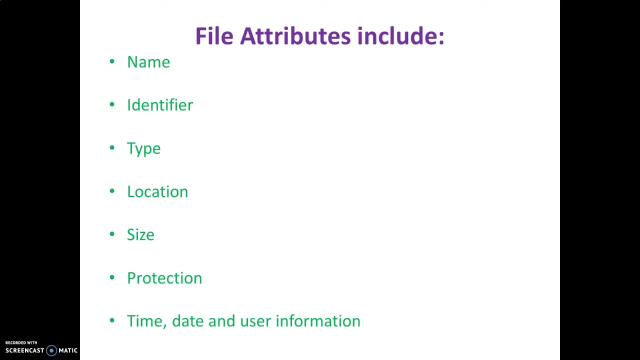 It is going to give me, Which Can only be read or write, or it can be execute, So that information later to the time, date and user information when the file was created, when it has been modified, So any kind of information related to the fight. 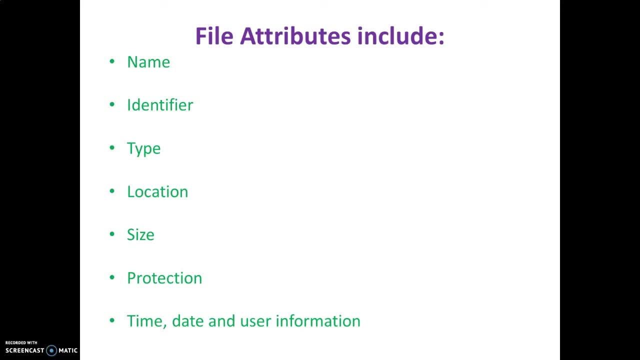 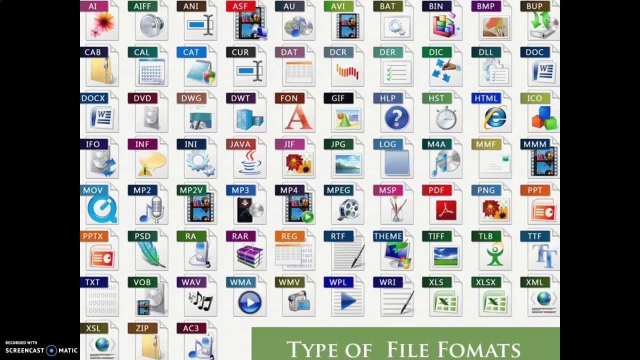 So these are all the different attributes which are included in the case of fight. So these are all the different formats of the fight. I think So many options are available today For the audio Video image simple document file we are having, Whether it is a source file or you can say object file, it is. so so many options are available. 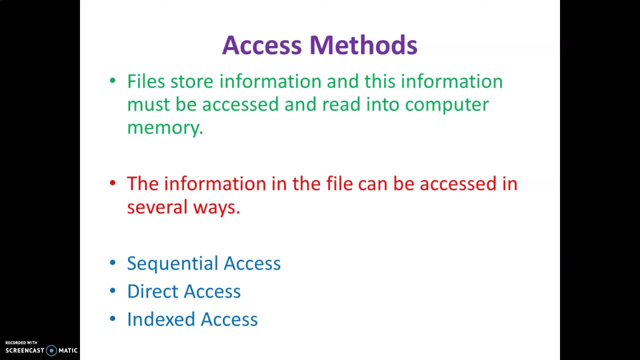 In today's world. So, then, very important Topic we are having is the access methods. so access method is basically the file stores Information, and this information must be accessed and read into the computer memory. So which means that Whatever the file we are storing, 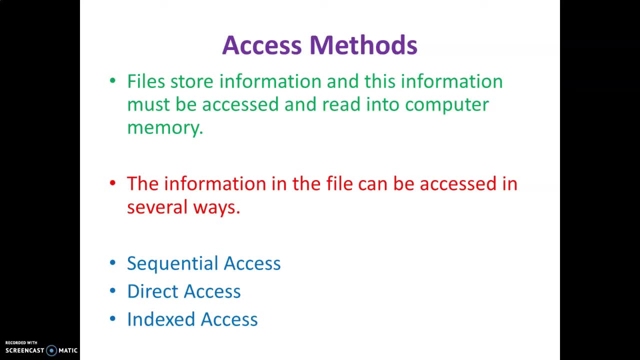 So these files we are going to access in the future. So basically, the information in the file can be accessed in three different ways. The very first one we are having is a sequential access, Then we are having the direct access And the last option we are having is the indexed access. 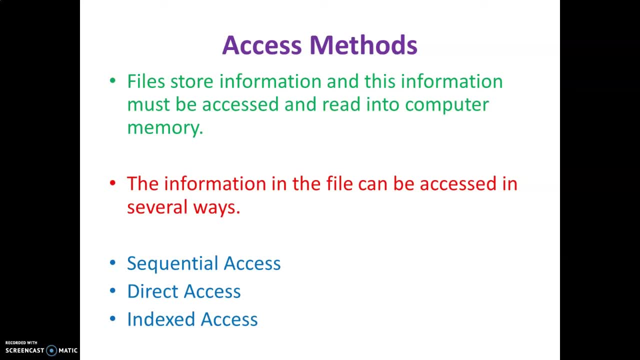 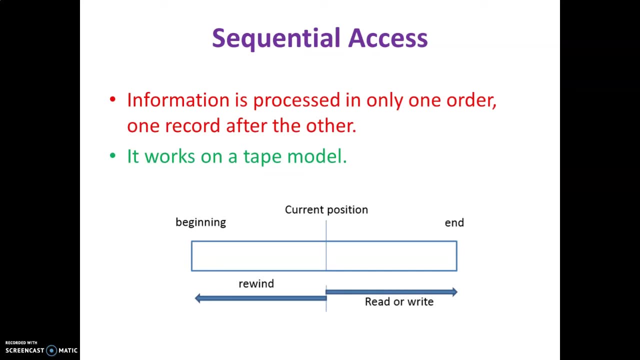 Let us see all these different access methods one by one. The very first one we are having is a sequential access, Sequential access. The name only says that in the consecutive manner, which means that the record we are going to read one by one means one after another. 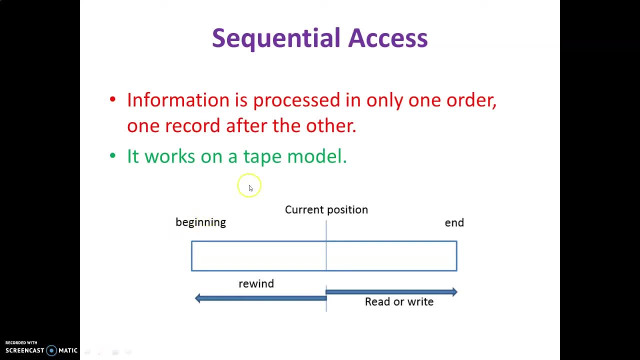 So it works on the model of the tape, like we used to have in the earlier time. So we used to have the cassettes A and B, which means that fixed data or fixed size will be given to us. So if I want to read, 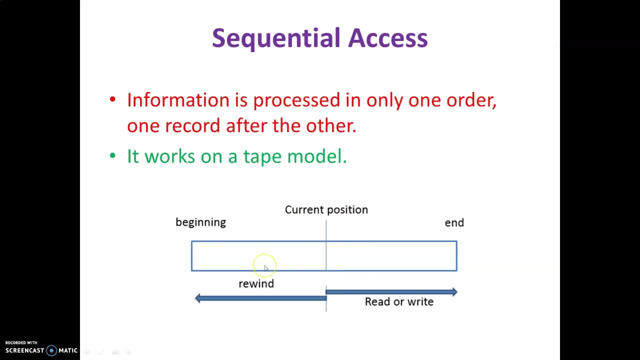 Suppose This diagram, only Suppose these are the different directions or different with the different operations, So read, write operations will be done. Suppose my current location is at this place. Suppose total 10 songs are available in my cassette, So after that I am suppose playing the fifth one. 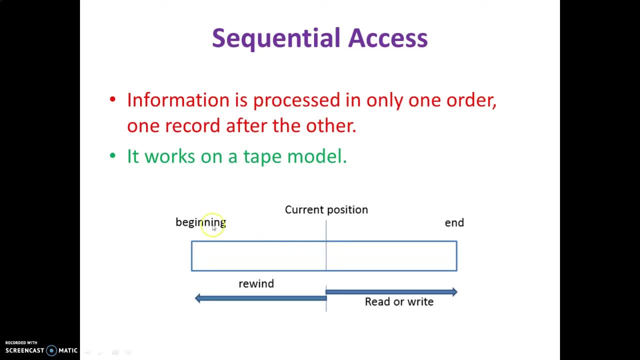 So if I want to read the first one, it means directly I cannot jump to the first song, which means that first of all, like we used to rewind, in that case First of all from the fifth position I will move to the fourth, then third, then second. 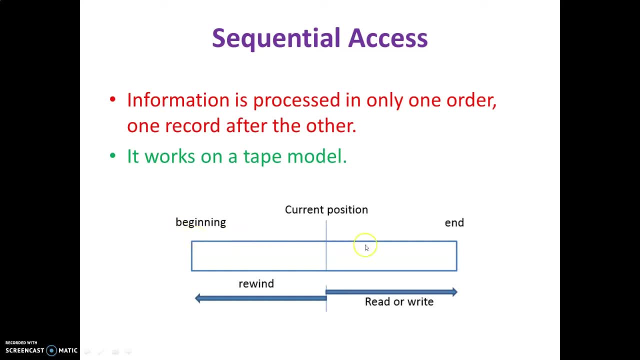 then I can read the first data. Similarly, if I want to read the eighth song so directly, I cannot jump to the eighth position, which means that first of all I will read the sixth, then seventh, then eighth, like this: This is how sequentially the data was read in the case of sequential access. 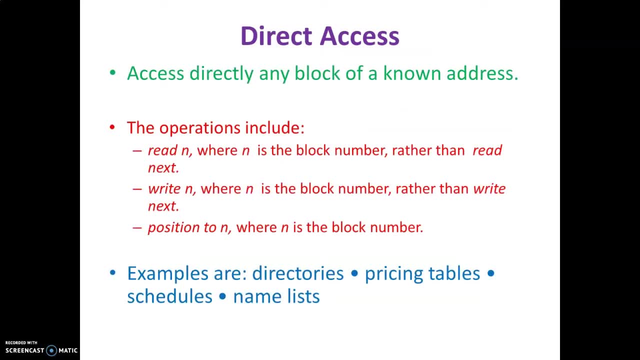 So then we are having is the direct access, Direct access. Direct access means now we were overcoming the problem of that sequence, which means that directly, whatever the record is given to me, I can directly jump to that record. So so access directly any block of an unknown address. 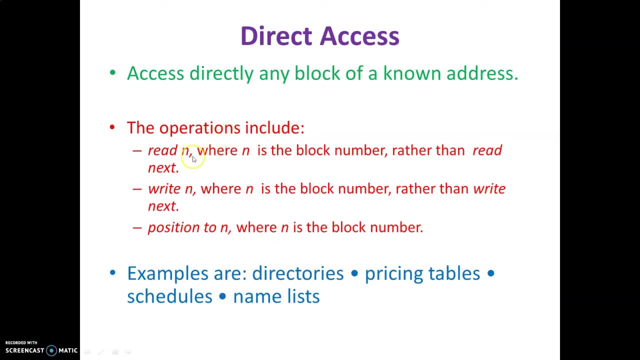 So the operations were like: read n. Now n is the number or the block number where I want to jump. Suppose I am at the fifth position. now I want to read the second, second song, second record. So what does it mean? Read two. 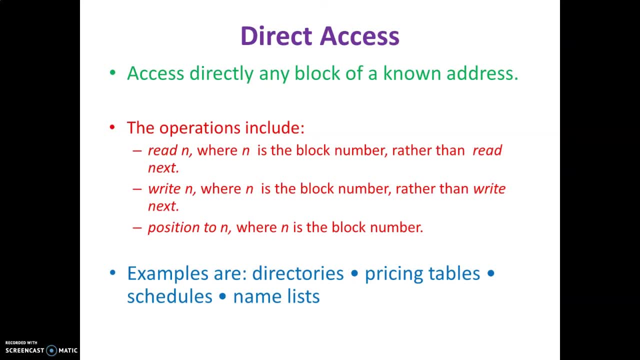 So from the fifth position directly I will jump to the second position. So then I'm having is the right n. So again, if I am on the fifth position, if I want to write further the eighth record directly, I will be giving the eighth value over here. 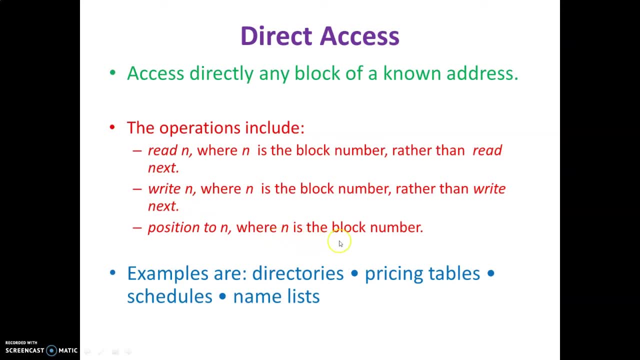 So so n what n represent over here, The block number, which means that direct block number or direct data can be read by jumping from the current location to that particular location. So real. so there is examples we are having like directories, price tables, schedules and name lists directory, I mean to say like phone directories we are having today. 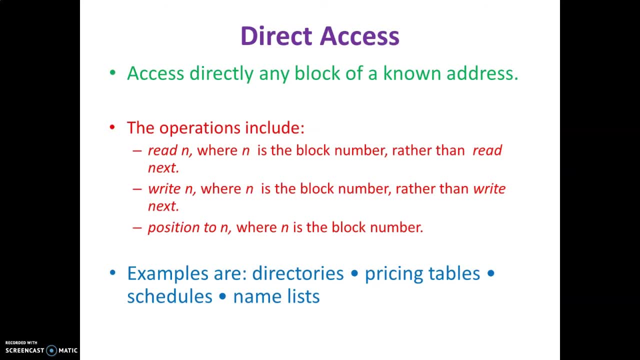 So, whatever the search you want to make, suppose I want to make a search related to the s character, So directly I will jump from, suppose, A alphabet directly to the record of s inside the phone directory. So this is how We are making the direct access. 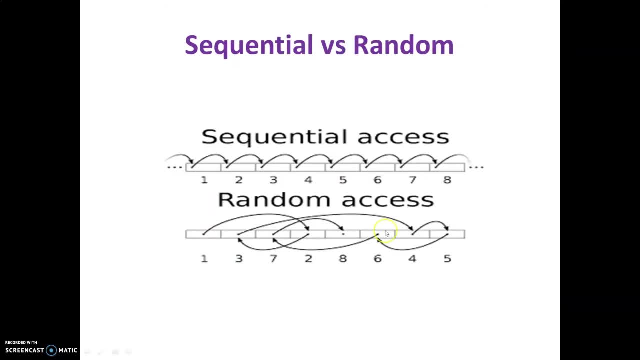 So this is a small comparison I have made in the case of sequential and the random. So see how data we can read in the case of sequential, one after another. Then, in the case of random access, see wherever you are. your current location is suppose at 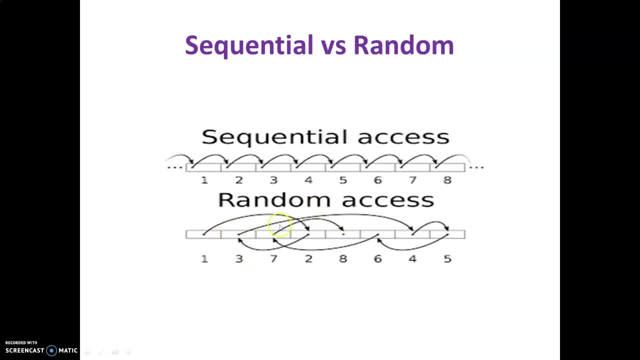 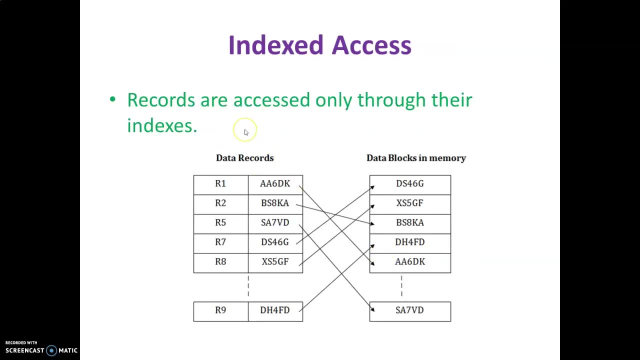 the eighth position if you want any another data. So you can jump from any location to any other location. So last one is the index access, which means that the cards are only accessed within the indexes. So this information we are having is related to the records. then all these are the indexes. 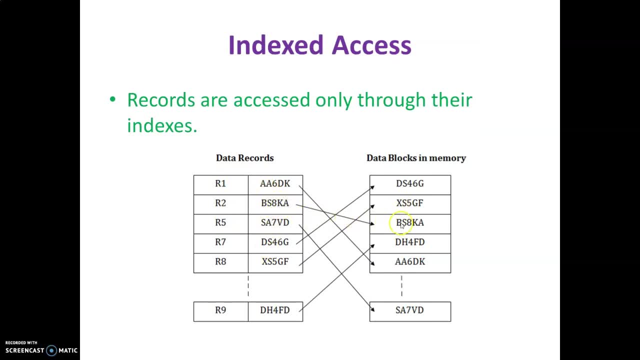 which means that they are going to point to the address inside the memory. Suppose, if I want to access this record two, where I am going to access this, suppose in the block number three, So which means that record two is available in the block number three. 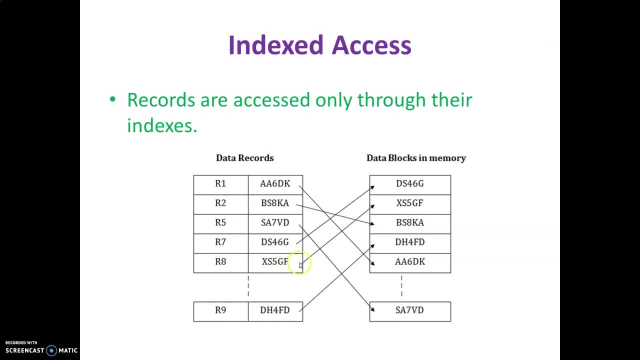 So similarly, record eight where it is available. So this index is pointing toward this particular block, block number two. So this is how index access work. So thank you so much. Thank you so much.